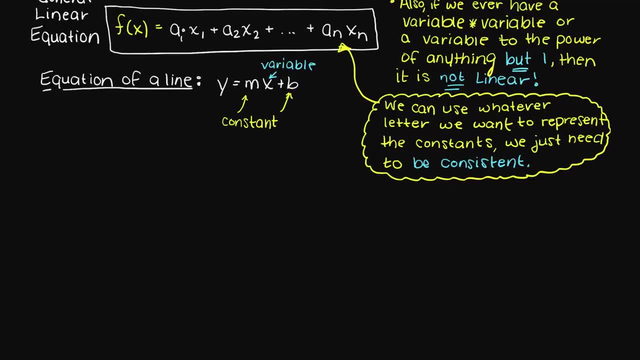 all of these are a constant or a constant times a variable. we know that our equation is linear, So you may ask: what would it mean to solve a system of linear equations? We will go through the methods of actually solving these systems of linear equations in future videos within. 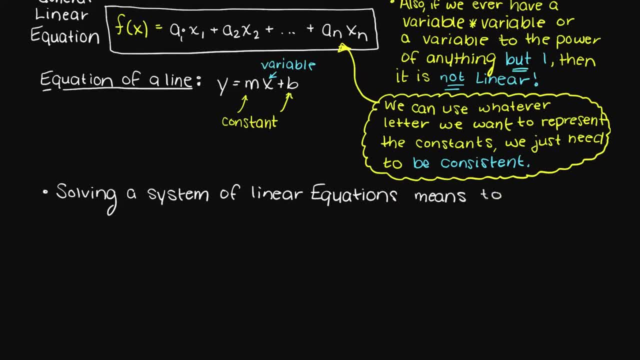 this playlist. For now, just know that solving a system of linear equations essentially means to find, and thus assign a value to each of your unknown variables. Because there is sometimes more than one solution to a system of linear equations, the total set of solutions that can solve our system of linear equations is called the. 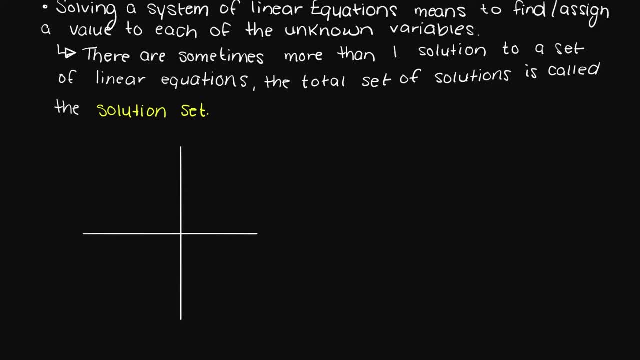 solution set. There are three possible solutions when solving a system of linear equations. Firstly, we could have infinitely many solutions, which occurs when our linear equations are on top of one another. Secondly, the system could have a single, unique solution, which is when our system of linear equations all cross at a single point. Lastly, the system. 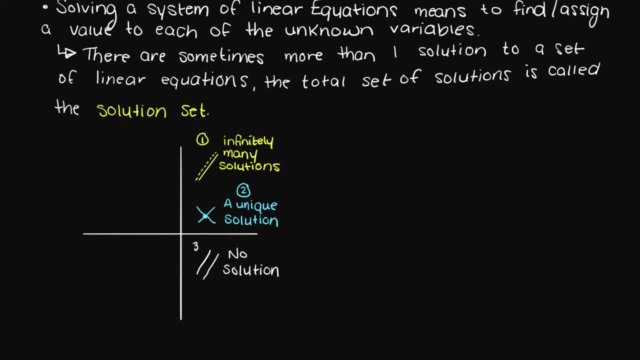 could have no solution, and this means that there is no possible point where all of our linear equations pass through. To more easily solve problems with relatively large numbers of linear equations, we can write the linear systems of equations in matrix form. So the way I think of this is that we keep an inventory of all of our variables within matrix A, The 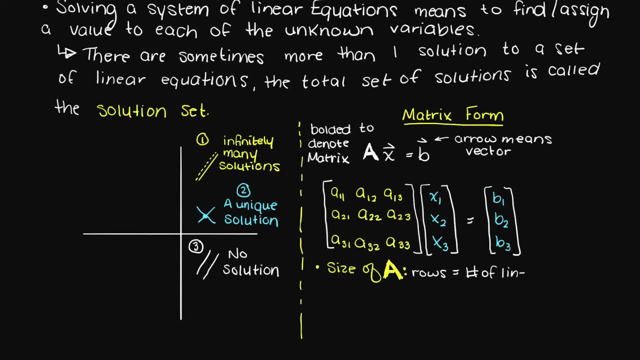 size of matrix A will be determined by the number of linear equations you have, which will tell you how many rows you need and the number of variables you need. This is the number of variables that will tell you how many columns you need In the matrix equation. our matrix A is multiplied by x, which is the column vector representing. 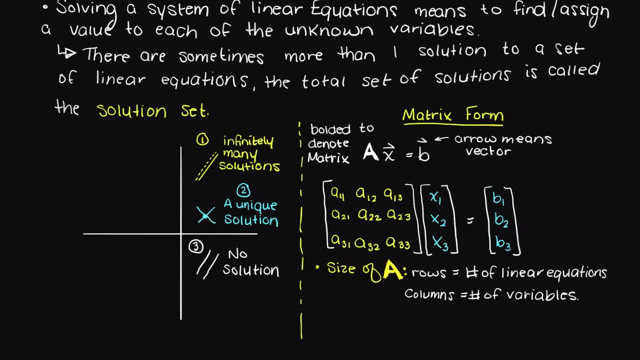 all of our unknowns. and this equals b, which is the constant vector, which basically means that it is just filled with some constant number, so 0, 10, 100, etc. This matrix equation can also be represented in an augmented matrix, which basically means the same thing. it just 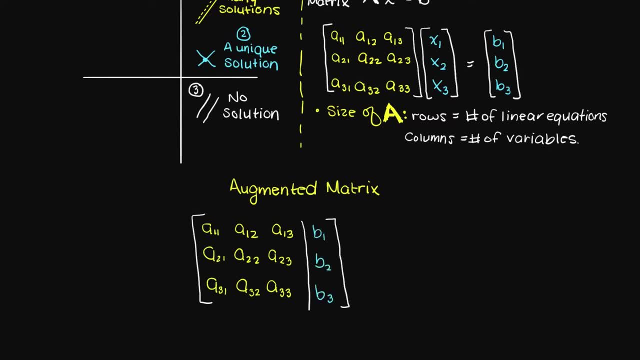 visually simplifies things. As you can see here, the augmented matrix looks very similar to the linear system of equations, but it is a little bit different in that it is a little bit more complex. An important thing I want you to note is that to solve a system of linear equations, you 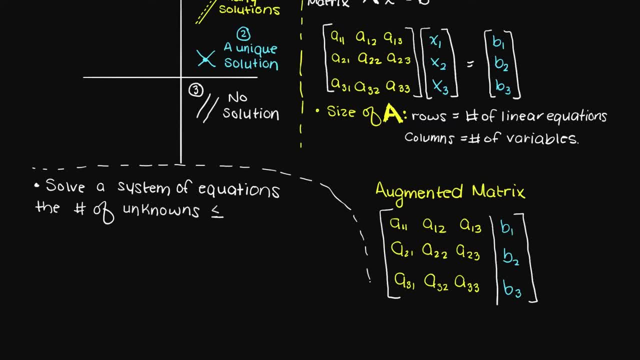 must have, at a minimum, the number of unknowns equal to or less than the number of equations you have. If you have more unknowns than equations, you will not be able to solve this system of equations. Throughout this course to more easily solve systems of linear equations: